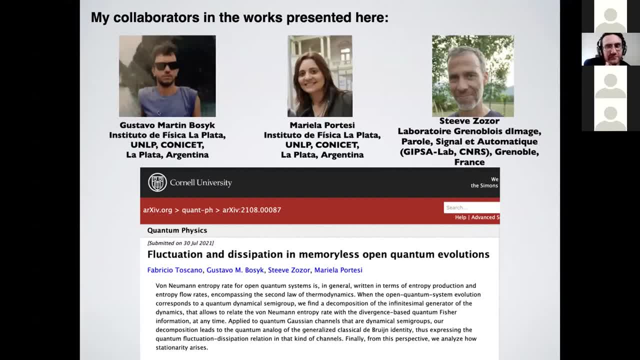 of the organizers of this conference: Professor Gustavo Martín Bosic and Mariela Portesi, that are from the University of La Plata, And Steve Saussure, that is from France, And you can see our work. that starts this collaboration started in the first conference that I attended in this series And well, it is in the archive. 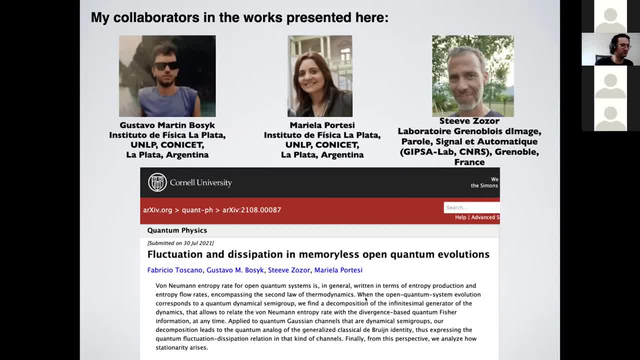 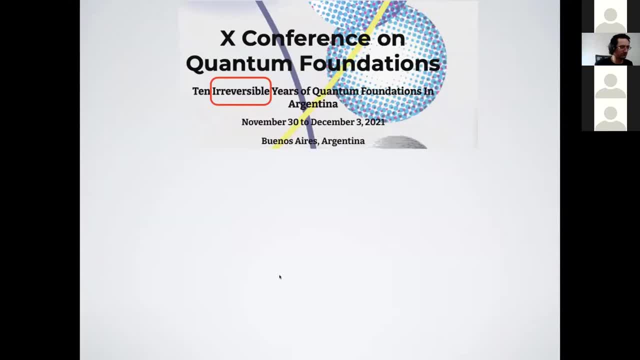 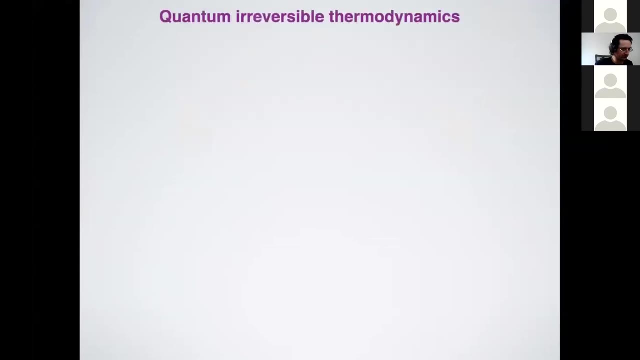 and this is the work. So I want to take the title of this conference that says that 10 Irreversible Years on Quantum Foundation in Argentina. I want to give you a brief motivation of our work that is based on quantum- sorry, quantum- irreversibility. 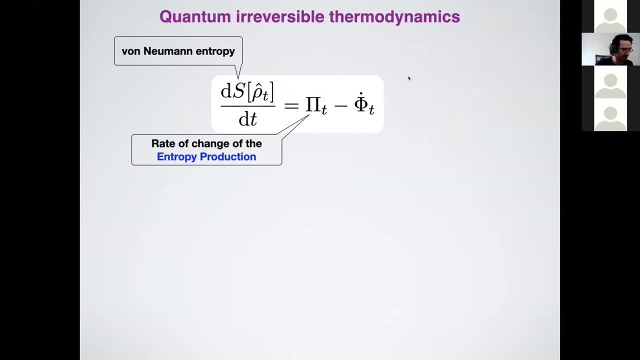 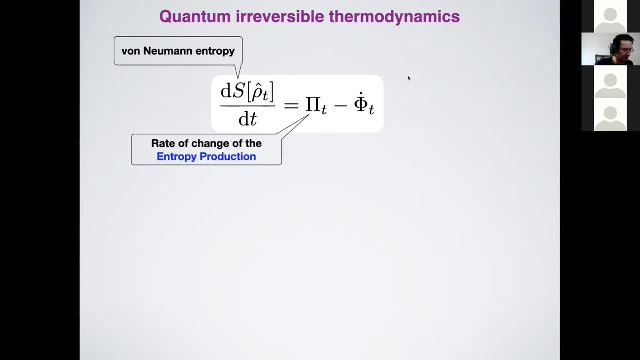 quantum evolution, the rate of change of the new economy? I'm not sure, but you said you got deceptive thinking. Dukt diesel Avatar. as you would imagine, that is basically farming 95, destiny for a based on in thermodynamics way of thinking. 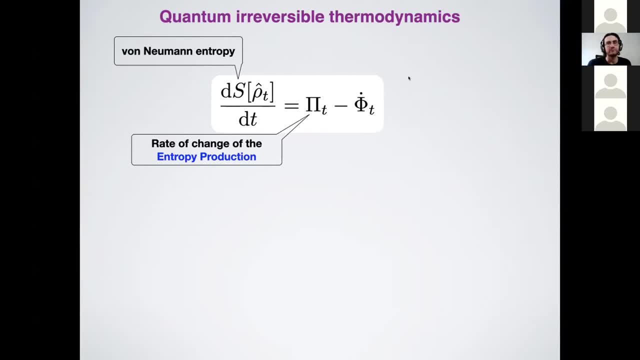 this rate of change is splitting in two parts. One is the rate of change of the entropy production and the other is the rate of change of the entropy flux. The second law of thermodynamics is just the statement that the first part, that is, the rate of change of entropy production. 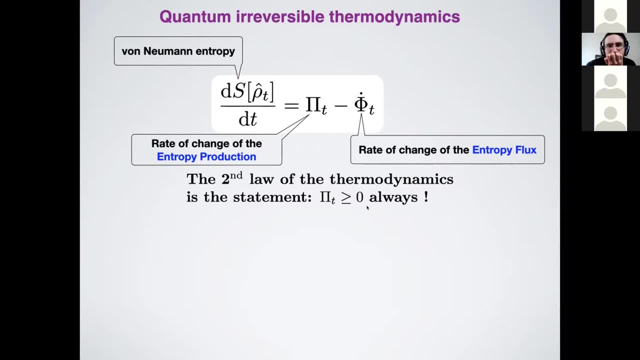 is always positive or zero. There is a big open question which is the general way to do this, splitting in a general open quantum evolution. but the problem is solved in several cases And at this time type of analysis gives a clue of how to analyze. 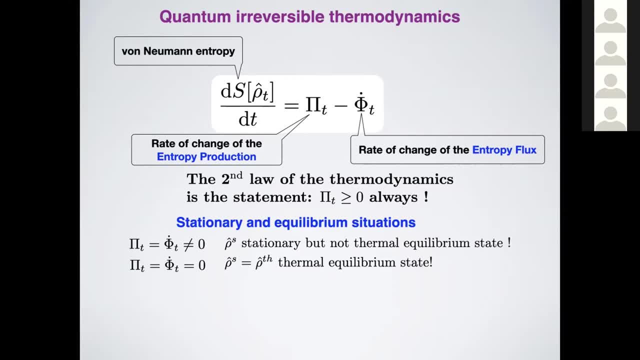 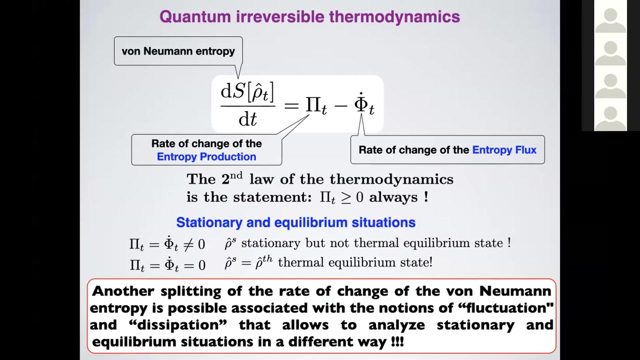 the stationary situations, conditions in open quantum evolutions, For example. the stationary situation is the balance between these two terms here And The balance, of course, but also each of these terms is zero. This corresponds to thermal equilibrium. OK, But I want to present here an alternative way. 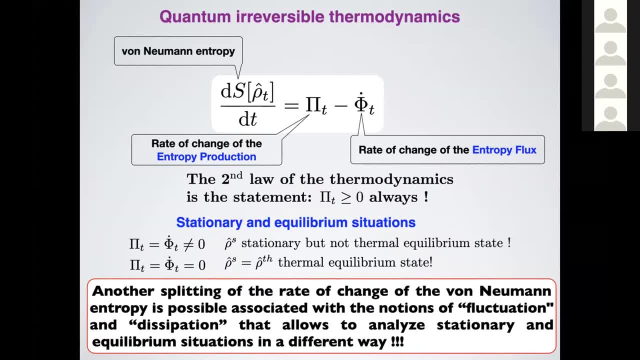 to, at least in a particular kind of open quantum evolution, but very important kind, And I will present another splitting of the rate of change of the von Neumann entropy that is associated with the notions of fluctuation and dissipation. And this new splitting allows to analyze the stationary 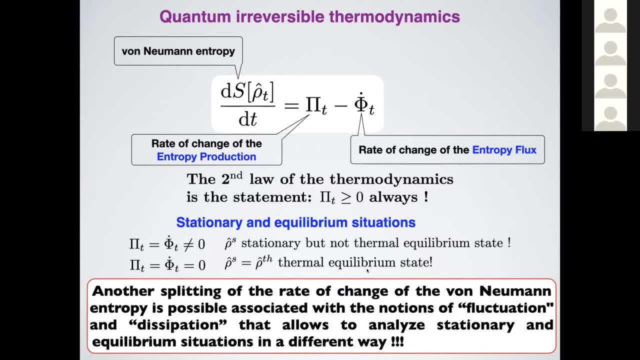 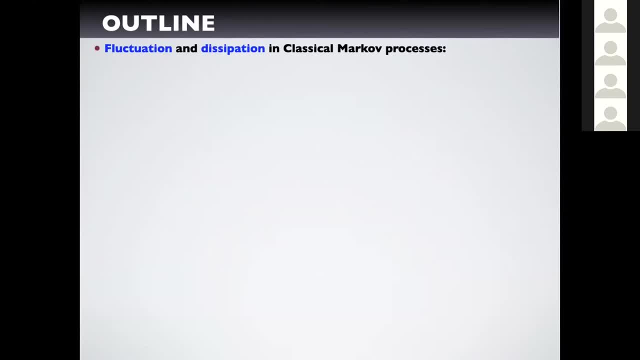 situations in a different way. OK, So this is the main motivation Of our work. So first I will introduce which is the notion of fluctuation and dissipation in classical Markov processes. I will talk about the additive, noisy Gaussian channel and how to generalize this very important channel. 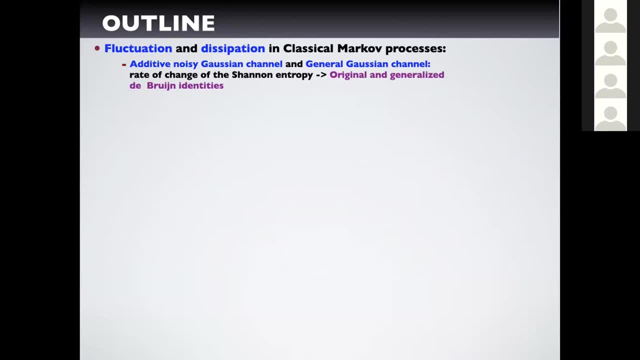 in a classical information theory to a more general channel that the Gaussian channels. And then I will Start to talk about quantum, open quantum dynamics and how to describe memoryless quantum communication channels that are continuous in time, And I will show that all of these kind of memoryless quantum 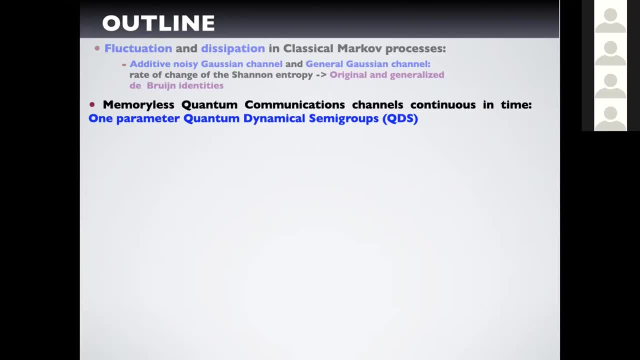 channels, continuous in time, are described by a one parameter point: Quantum dynamical semigroups. Then I will present the main result of our work, That is, a new decomposition of the infinitesimal generator, nonunitary infinitesimal generator associated with this one parameter. 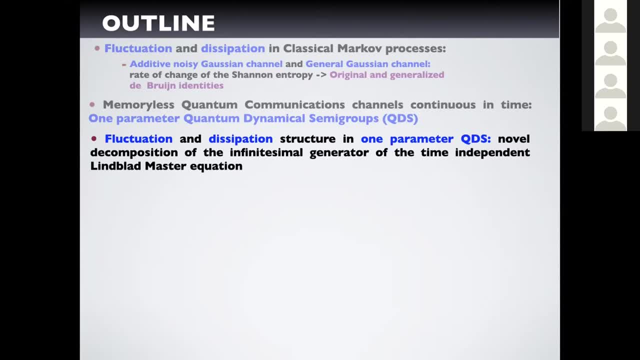 quantum dynamical semigroups. that verifies a limit blood type of master equation. And then I will show how this decomposition of the infinitesimal generator allows to write the rate of change of the normal entropy in a particular way where you can identify the fluctuation and dissipation terms. 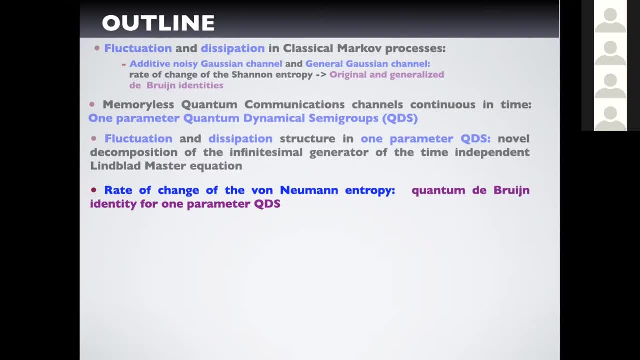 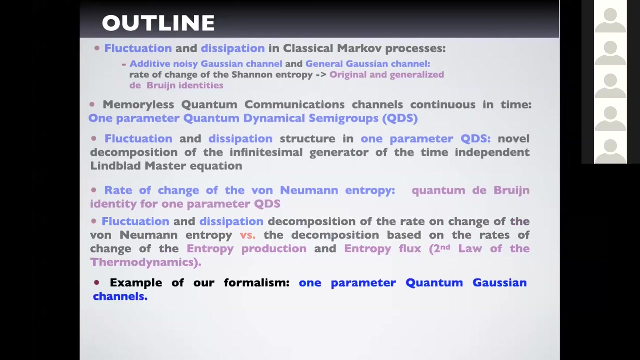 And this is the quantum analog of the classical, very well known Debrushing Identity that appears here in classical Markov process. Then I will compare our approach with the approach of the thermodynamic universe, of quantum thermodynamics, And I will give an example in a one parameter channel: quantum Gaussian. 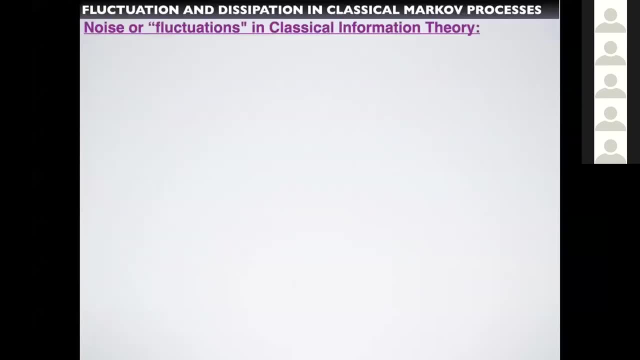 channels. So let's start with Noisy fluctuation, classical information theory. The most important type of channel here is the additive noise Gaussian channel. That corresponds appears in very natural random processes that are viewed as a large sum of noises. sources of noises. 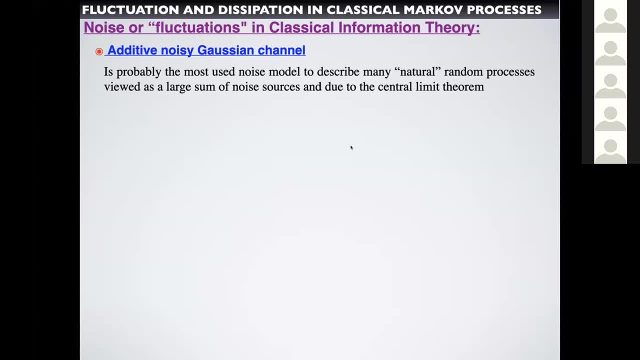 And if you combine this with the central limit theorem, you end up with this type of a challenge. So the channel is is you have a random variable and you combine with a noise that is described by a normal distribution, random variable, And this square root of t is the strength of this noise. 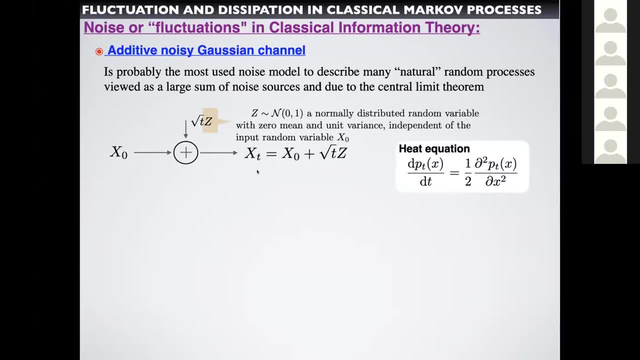 Okay, So the probability distribution of the random variable at the output of the channel verifies the very well known Heat equation. Okay, So the quantification of the of the fluctuation or noise in this channel is given by the original, the classical debris, debris identity that was proven for by a stamp in 1959. 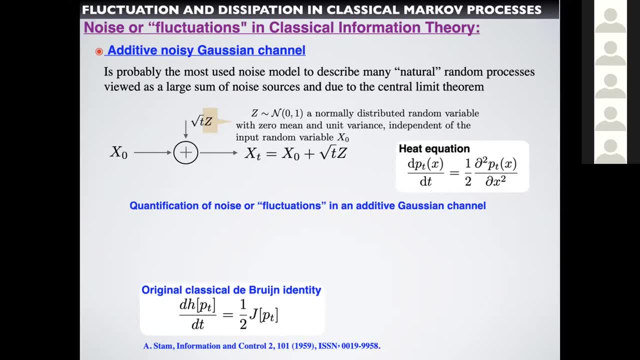 And is the rate of change of the channel and the rate of change Of the channel Shannon entropy here Okay, And this rate of change is proportional to the efficient information. This efficient information is The so called Fish information associated with displacement. 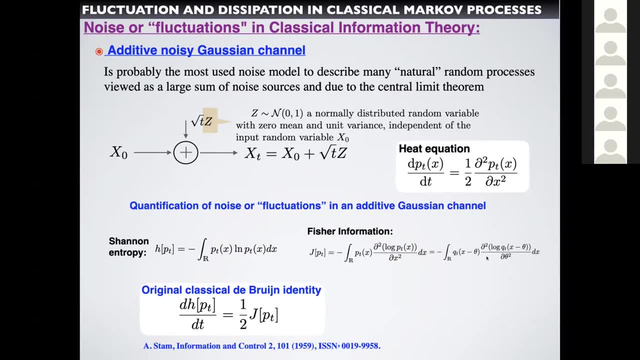 Where you can Is This displacement depends, like in any fish information, by a parameter, Tita, But this parameter, Because he's At this Displacement, Disappears, And This type of fishing information is also known as unparameter fishing information. 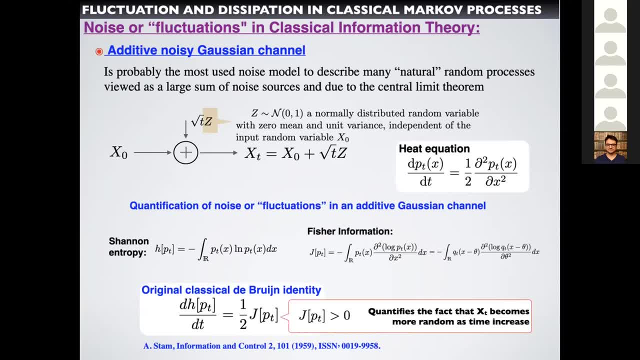 Okay, And this quantity is always positive. So This classical debris identity Only says that the quantified the fact that This random variable, Because becomes more random As time, increase. Okay, So The generalization of this type of 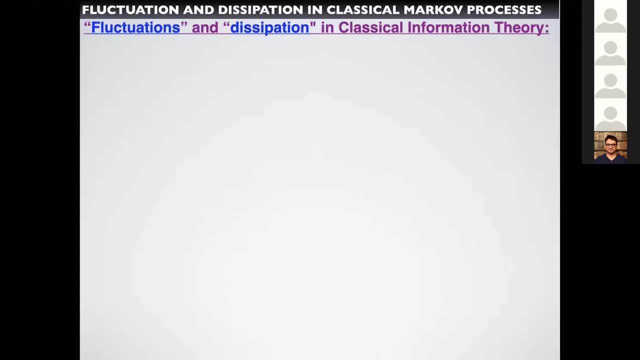 Channels in classical informational theory Is Given by the so-called focal plan channels That correspond to me, Dimensional Channels That are modeled by Launching on forces That are described by Stochastic differential equations And The more. 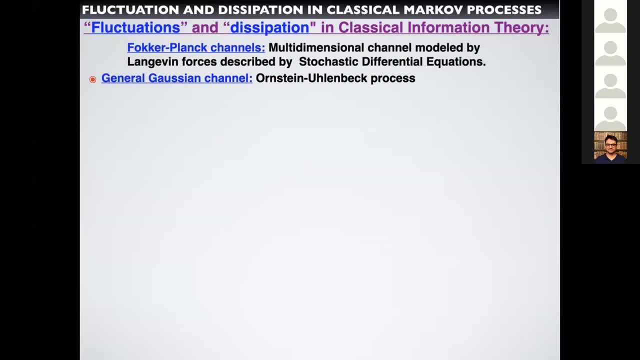 Important Type of These channels Are the so-called General Gaussian Classical channels That correspond to Einstein Eulenbeck Processes. These Processes Are described by: This is stochastic Equation. The first, Then, Is the 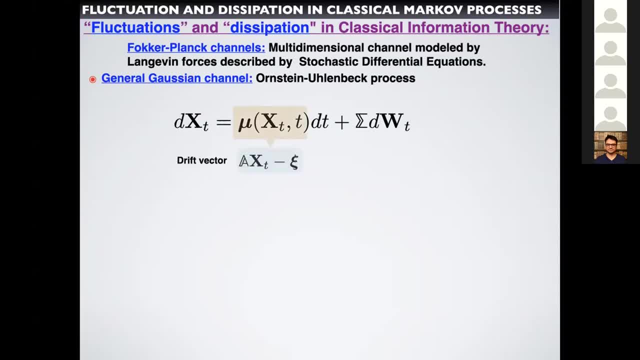 Drift vector. Okay, So This Stochastic Here, This X Is a vector, That is, The Multi-dimensional Random variables, And The Second Term Of the Financial Question Is the. 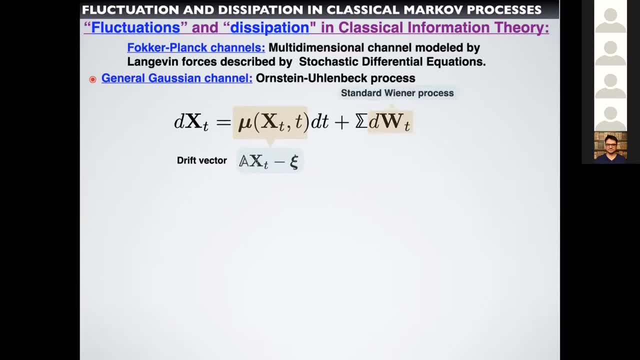 Standard Binary Process That Is Characterized By This Matter Here That Is Known As Associated With This Vector Of Random Variables. Verifies A Linear Focal. 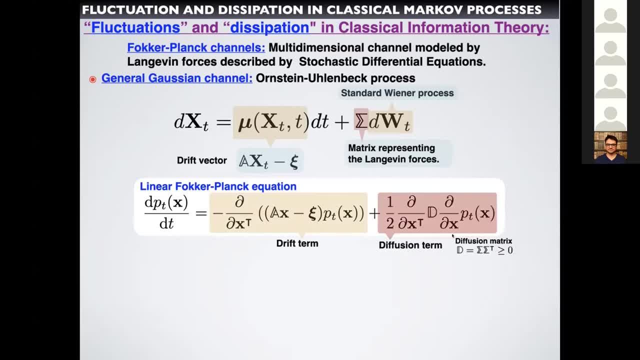 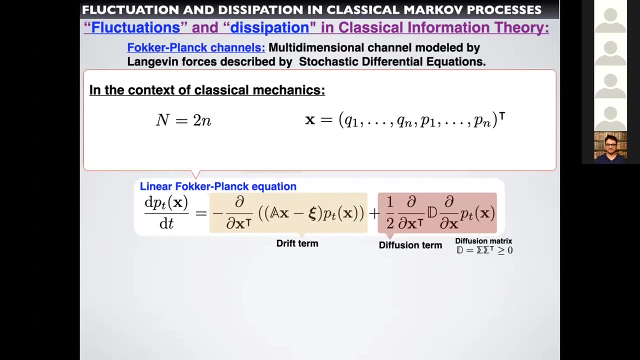 Plan Equation. Here Is The Linear Focal Plan Equation, Where The First Time Is The Drift Term And In The Case, For Example, When This 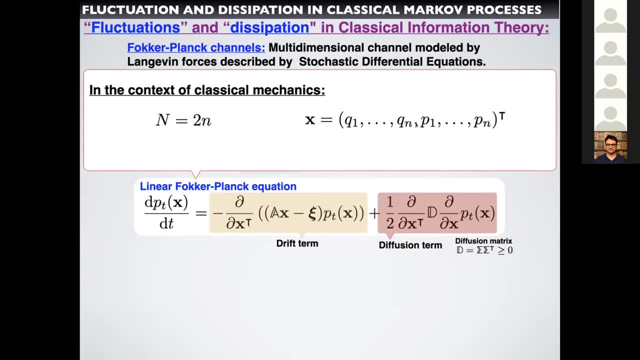 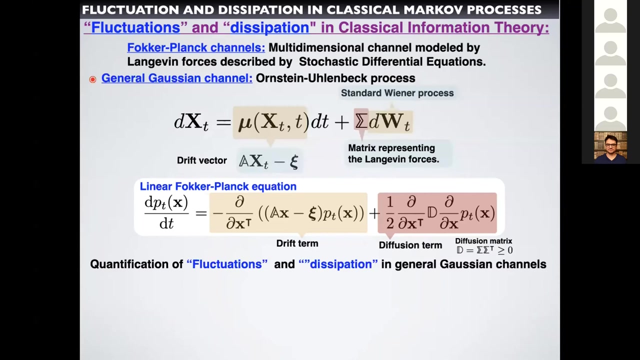 Random Variable X Is Just Face Space Variable In A Classical Mechanical System. The Typical Example Of In This Case Is The Linear Focal Plan. 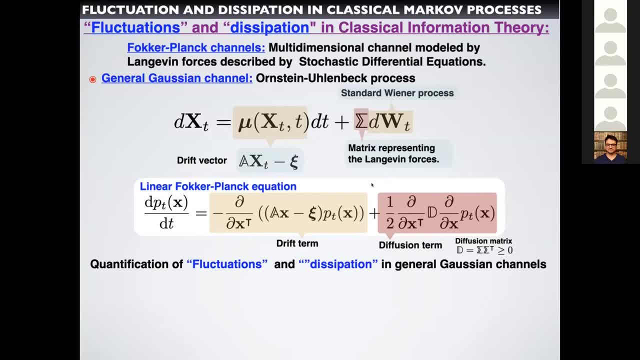 Equation And The Quantification Of Fluctuation Anticipation Associated With This Focal Plan Equation Is Given By This Generalizing Classical Identity That Was First. 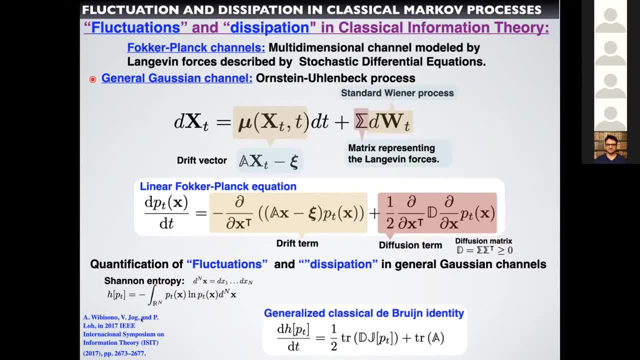 Written With This Type Of Log And This The Brewing Identity. The First Term Is The Contribution Of The Fluctuation. Here Appears The Diffusion. 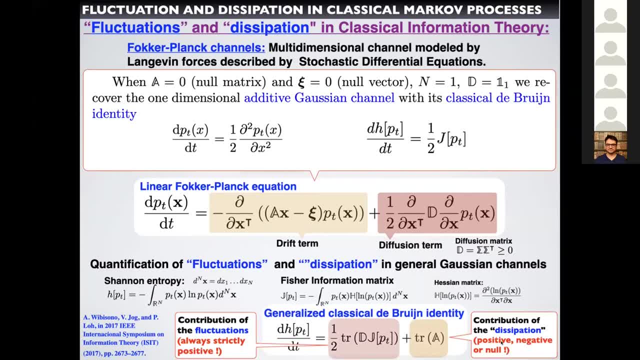 Matrix And This Diffusion And Also The Matrix Of The Diffusion And The Second Term Could Be A Positive, Negative Or No Okay In The 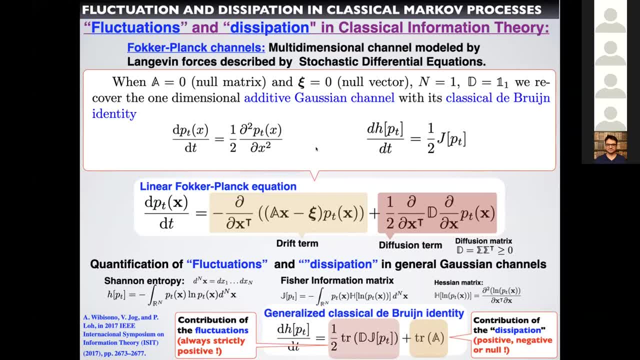 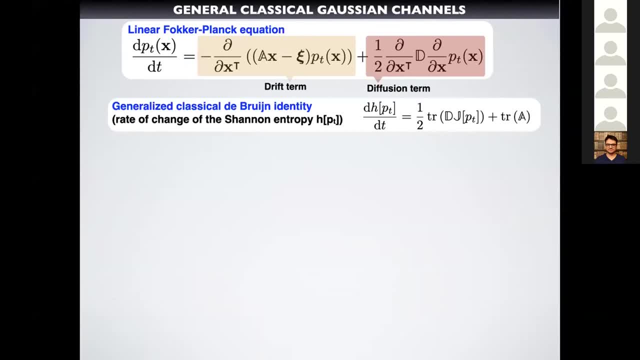 Case Where You Don't Have A Matrix. In One Dimension You Recover The. A Deep Look At This Structure Of The Generalized Classical Degreen. 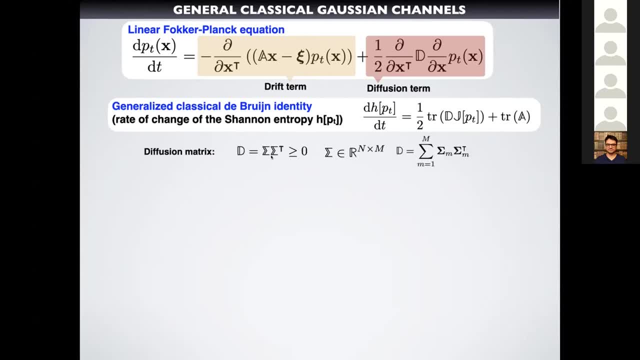 Identity. Okay, So The Diffusion Matrix Is Written In Terms Of This Matrix Of Langevin Forces And Because This Is Using The Columns Of The 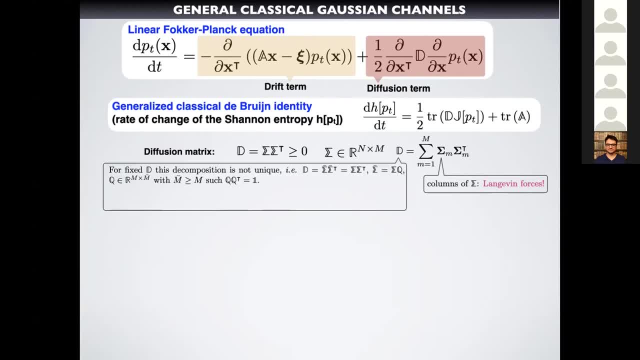 Matrix Of Langevin Forces. Of Course, This Composition Is Not Unique. You Can Use Any Langevin Forces That Are All Described In This Way. 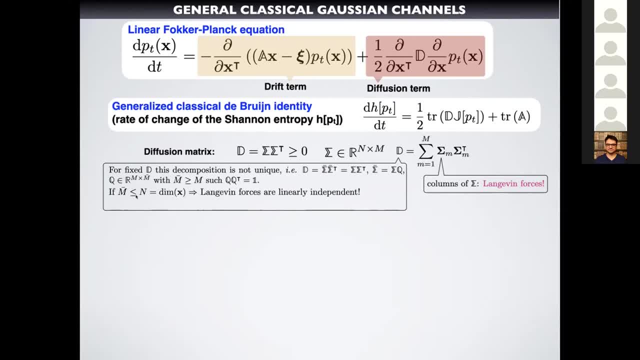 Is Less Than The Dimension Of The Random System, Then The Langevin Forces Are Linear, Independent And If You Have More Columns Are The Langevin. 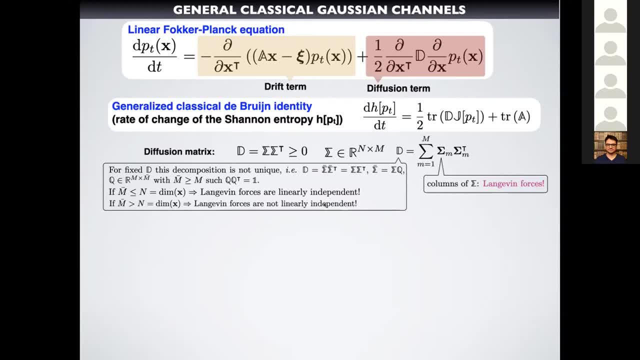 Forces Are Not Linear And Choose Any Description In Terms Of Langevin Forces. That For A Given D, Okay, So Using This Decomposition Here, It 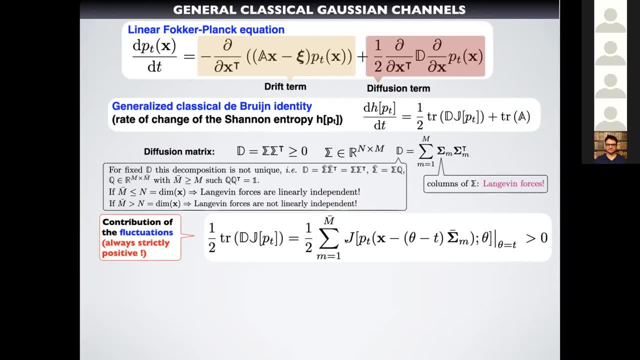 Is Easy To See That This Trace Of Probability Distribution And The Displacement Is Given By This Langevin Forces. Okay, For The Second Time That. 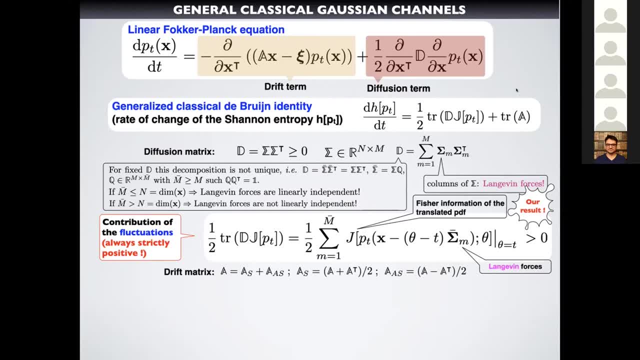 Is The Drift Matters. Here You Have A. You Can Decompose This Drift Here As A Two Type Of Forces. One Is The Antisymmetric. 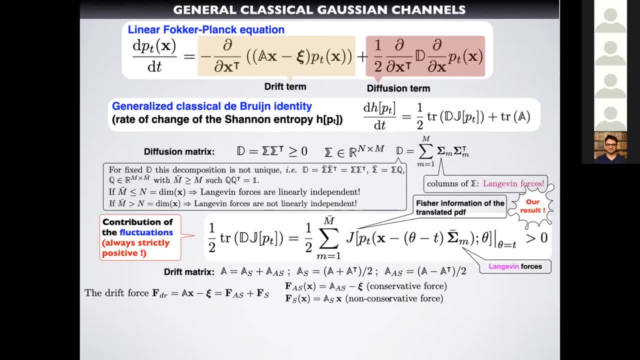 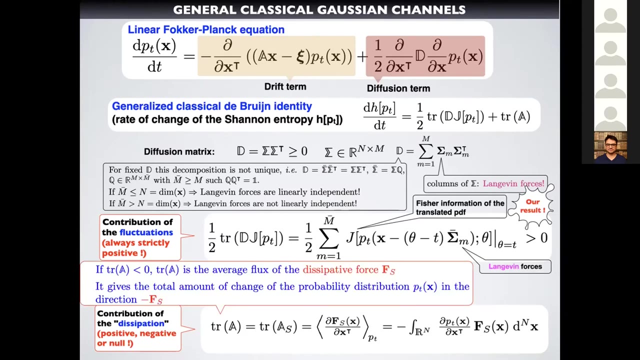 Part Of The Pathetics That Correspond To Conservative Forces, And It Is Easy To See That The Conservative Forces- And This Trace Here Is Just 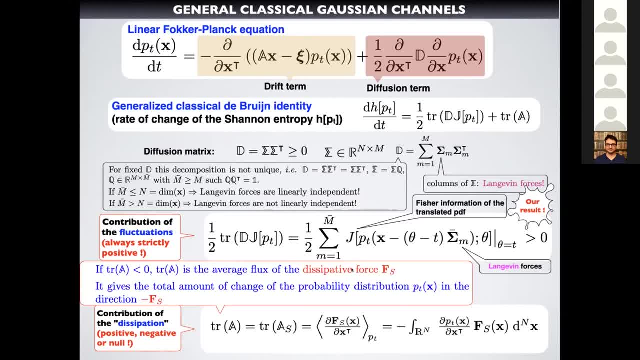 The Average Flux Of The Deceit, The Sympathy Force That Gives The Total Amount Of Change Of The Probability Fusion In The Direction Of: 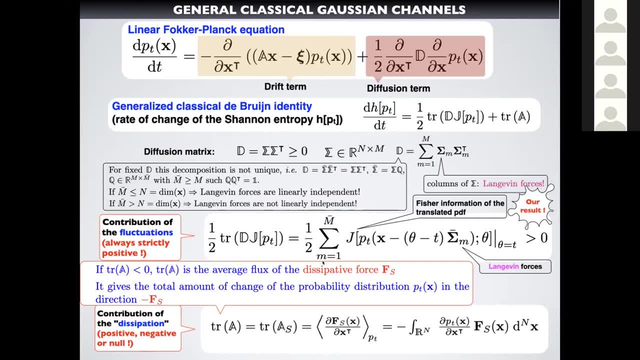 Course, Because, In The Situation, This Contribution Of The Situation Must Contrabalance This Average Flux Of The Deceit Deceit Force. So Let's. 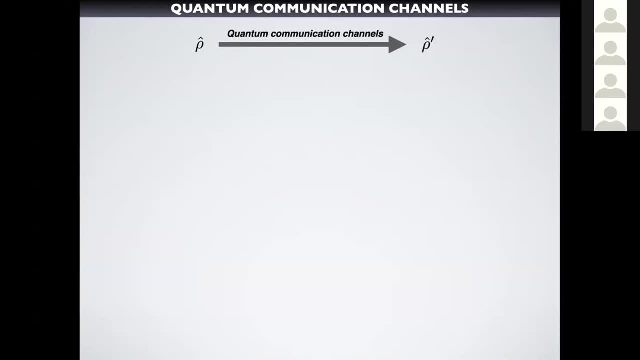 Now We Want To Apply These In A Classical Mark On Processes In Focal Plan Channels, In Classical Information Theory In The Quantum Domain. So 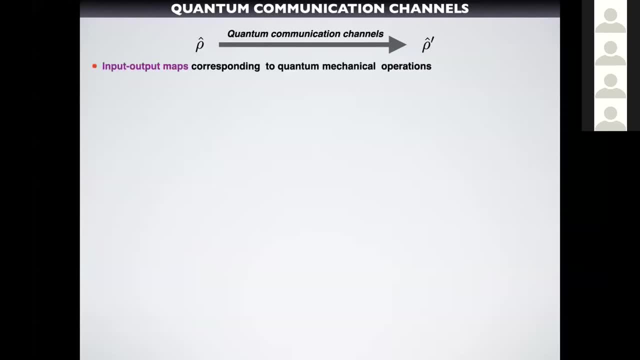 Let's Start Talking About In General What Is A Quantum Channel A? This Operation Is Shedding A Picture, A Correspond To Maps That Are Completely 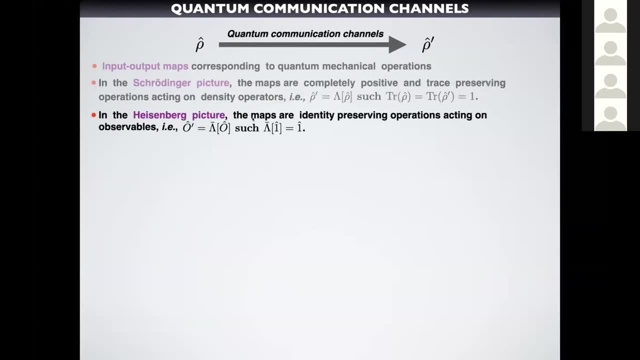 Positive And Preserving That Act On Density Matrix Here And Our Preserving A In The City Of The Trace Of The Density Matrix In The. 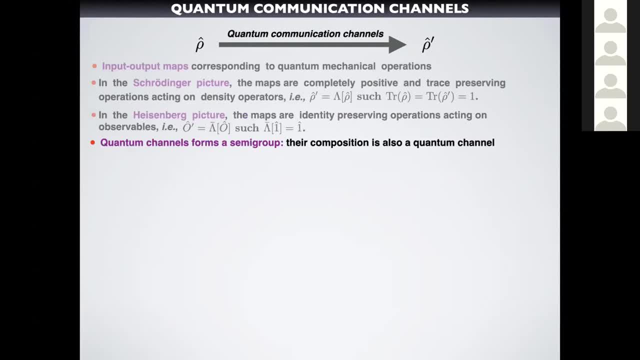 Hasn't Been Correspond To The Preservation Of The Identity. Okay, This Will Be Important In General. Quantum Channels, Quantum Of Of Time In This Composition. 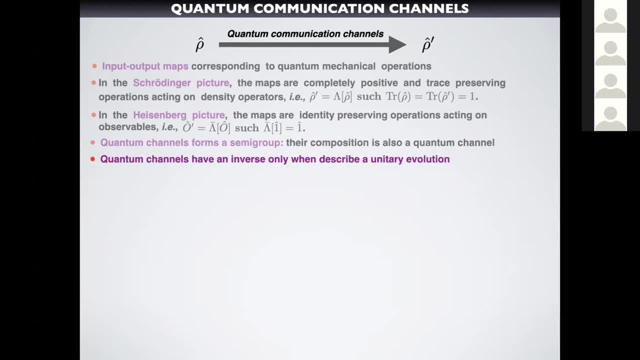 So It Forms, As Any Group, A Quantum. Channels Have An Inverse Only When Are Described By Unitary Evolution. Okay, So The Most Common: 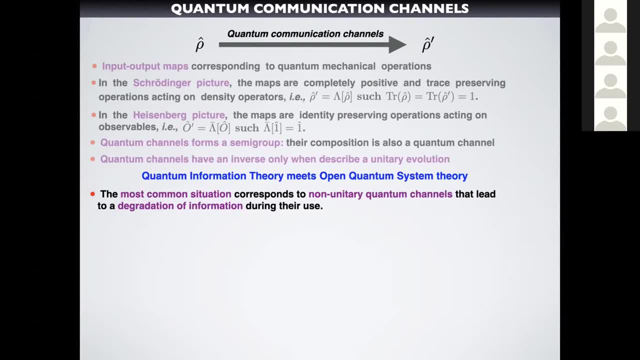 Environment Affects The Evolution, So The Most Common Situation Is To Have A Non Unitary Quantum. Channels Gives The Gradation Of Information During Their 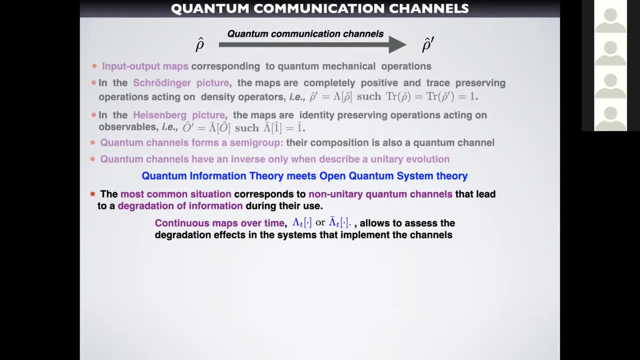 Use And In Order To Your Implementation Of The Channel, And This Gives The Necessity To Use Maps That Are Continuous In Time. Okay, And 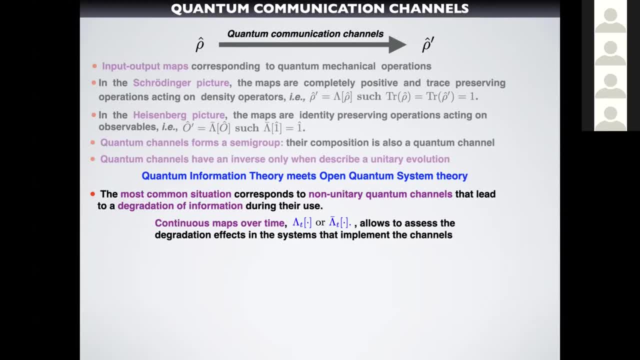 When You Use This Type Of Maps To Describe The Quantum Channels A, You End Up With An Evolution That Is Describing Always By The 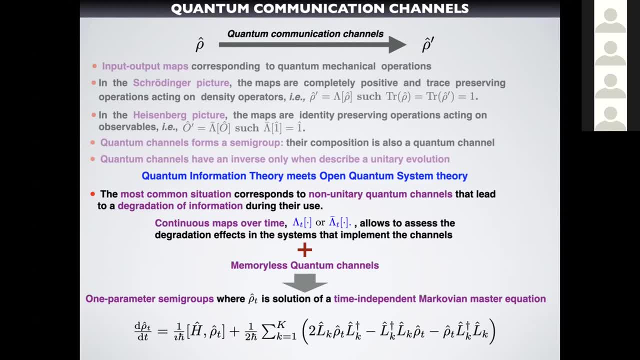 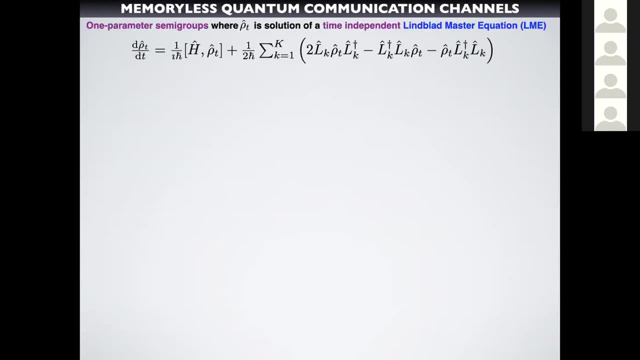 Time. Independent Master Equation And Whose Solution Are One Parameter- Semigroups, So Let's Use Limblad Master Equation In General. Okay, And These Are. 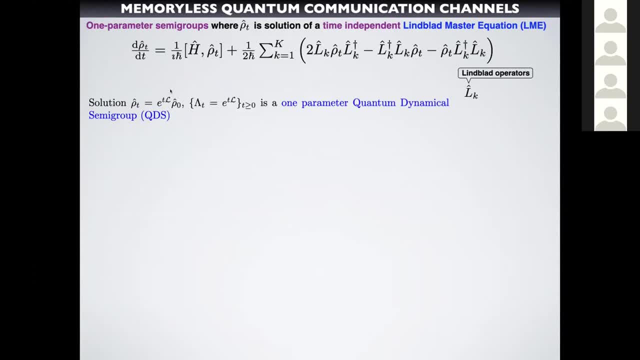 L Are The Limblad Operators And The Solution Is Given By This Map Here. That Is A Dissolution At This Solution And This Is 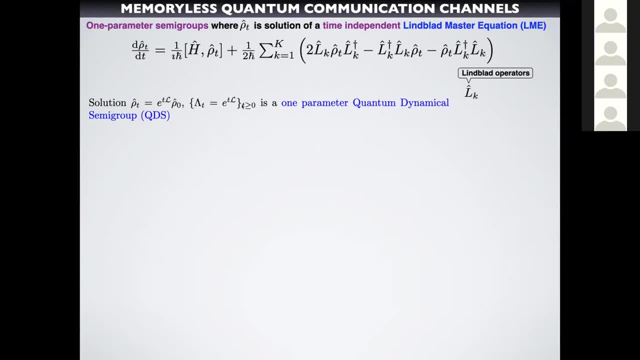 Also The Case For Very Important Channels In Continuous Variable System That Are Corresponding To Linear Master Equation That I Will Show You In A 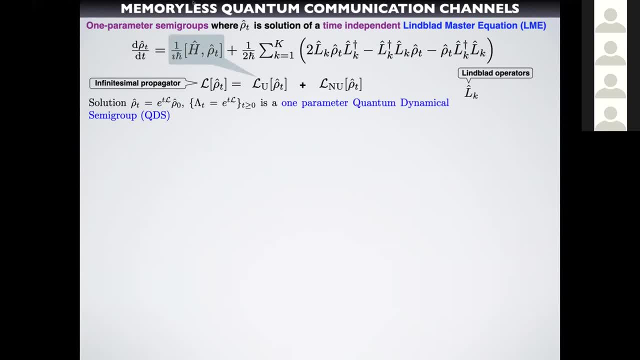 Definitive Propagation Sitting With. You Need The Revolution, And The Second Is The A City Within. So We Answer To This Question That Which: 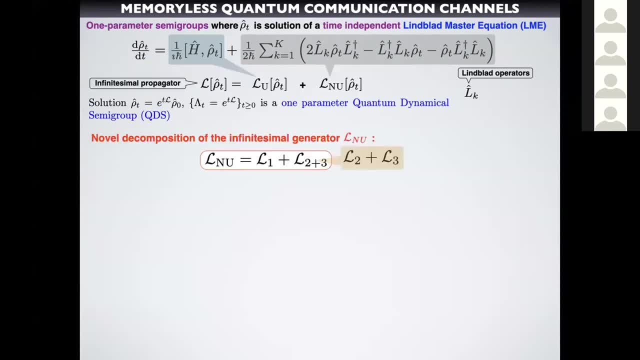 Is. The General Structure Of The Nonunitary Evolution Can Be Split In This Way: Where Appears Three Super Operators. Here Are Written These Super Operators. 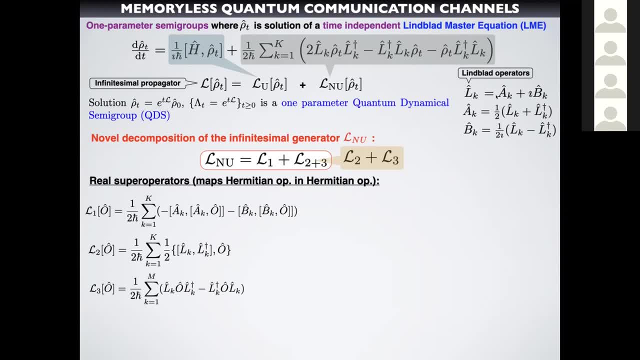 In Terms Of The Limblad Operators Where We Use, For A Part Of The Of The Arbitrary Limblad Operators. So The First, The L. 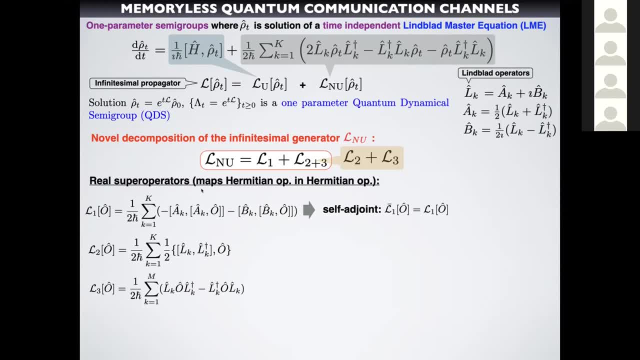 One That Appears Here. All These Super Operators Are Real. It Means That Maps Hermitian Operators Are A Scalar Product, Okay, And This A Open. 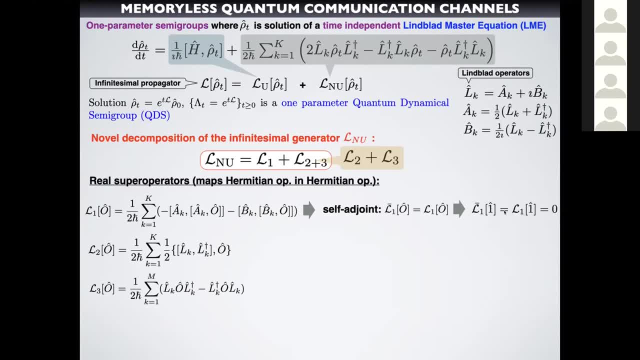 A Cell Self Joint Operator A Verify This And This Means That The Map That, If You Use Only This As You Find Here, Is I. 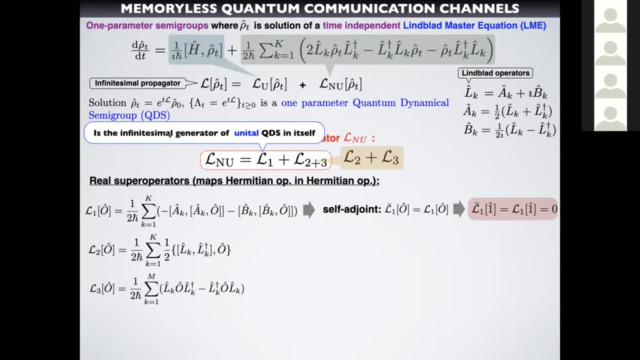 Are A Possible And Quantum Dynamical That Is Unital. Okay, The Other Two And And, Two Here And Three That Combining In This Way. 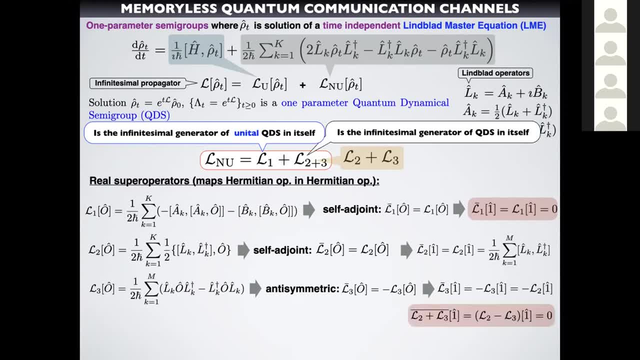 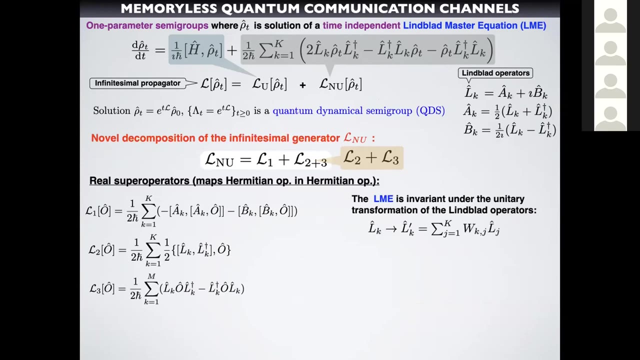 A, And The Combination Of Both Also Gives A, The A Possible If. If You need This In Itself, Okay, This Composition, It Is Very Well. 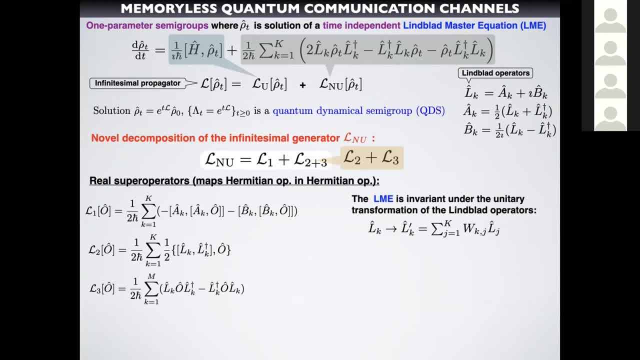 Known That The Symmetry That Must Be Verified By The Limblad Operators Is This One Where You Can Apply Any Unitary Matrix Here To 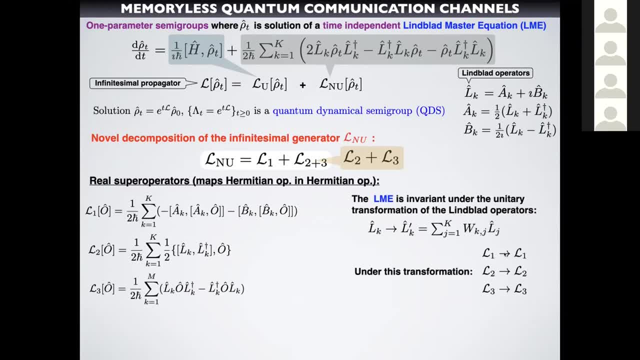 The Limblad Operators To Obtain Another Limblad Operators That Is Not Affected By This Type Of A. The Other Symmetry That The Limblad 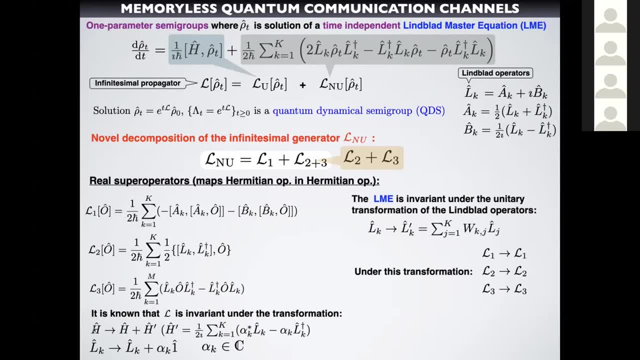 Operators Must Verify. Is This One Where You Change The Limblad Operators In This Way And This Symmetry To Our Composition? You See That. 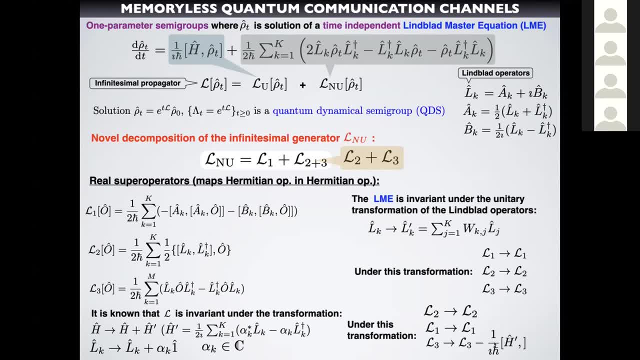 L1. And L2. Are Invariant And L3. Only Change, But In A Unitary Way. This Means That Appears Only A Contribution, That Is. 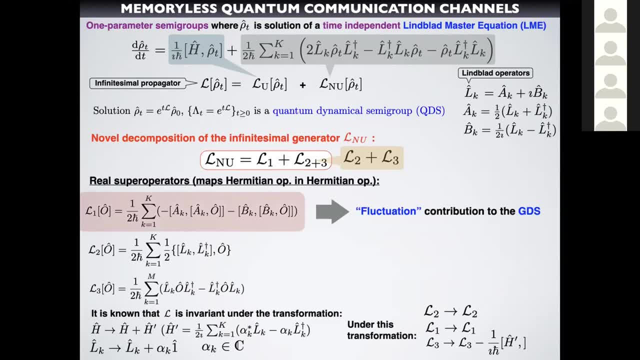 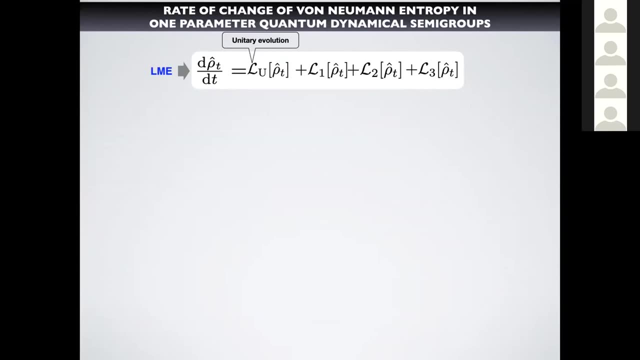 A. I Will Show You That The First Part Of This Composition Is Associated With The Fluctuation Contribution To The Gaussian Dynamical Semi Loop. 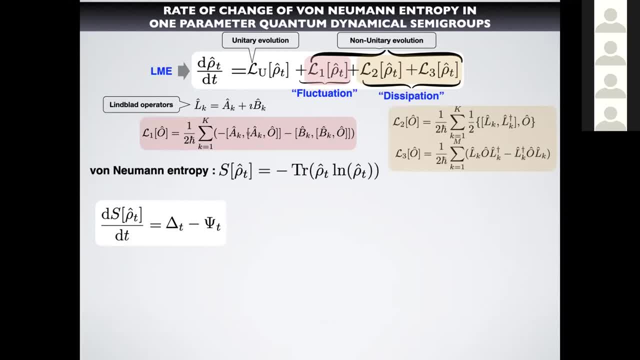 And The Other Two To See A How This Is Associated With Fluctuation, Dissipation. Let Us Calculate This: The Rate Of Change Of The. 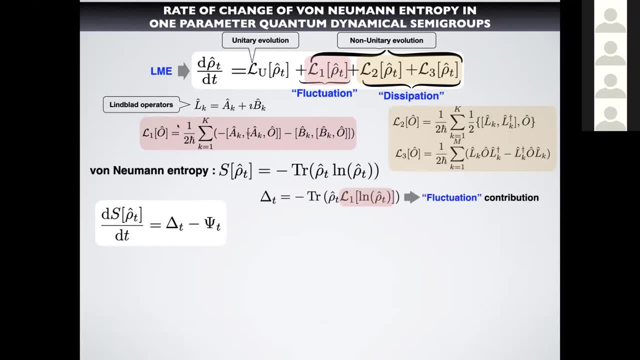 Monomer Entropy That Can Be Split In This Way, Of The Density Operator That All, Here And Here, You Must Put The Self Joint Of. 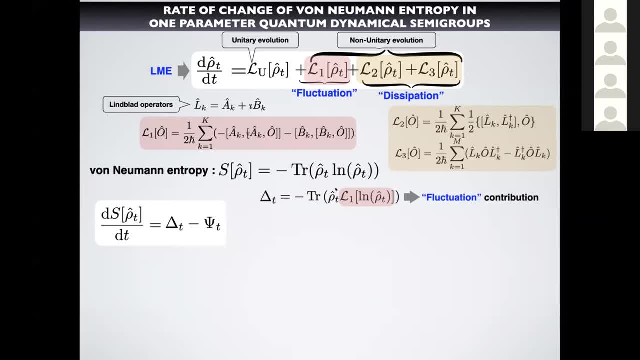 L1. But Because It's Self Joint Appears L1. So This Term Here Using This Other Time, Is You Must Put The Other Part Okay. 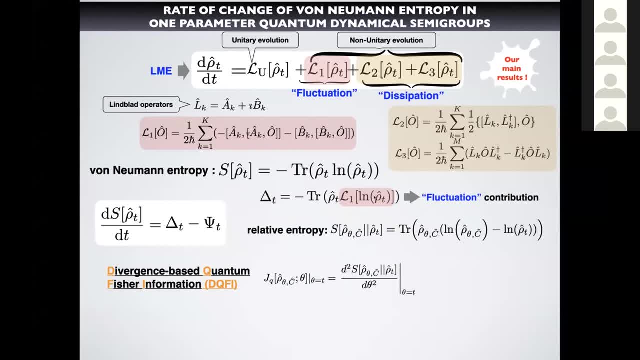 So This, The First Part Here, Can Be A Written Using This Relative Entropy That Is Written Here And The When You Use This Type. 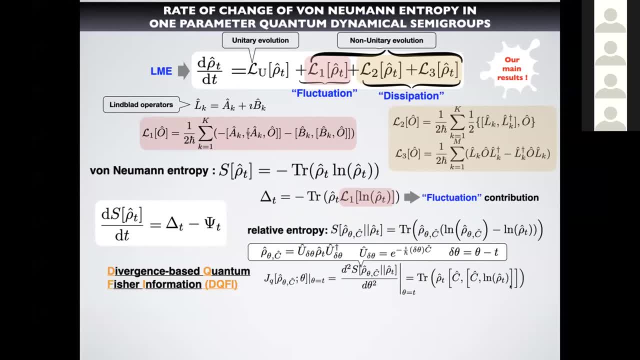 Of Evolution Here. It Is Easy To See That Have This Structure Here With Respect To This Double Commutator That Is The Generator Of Information. 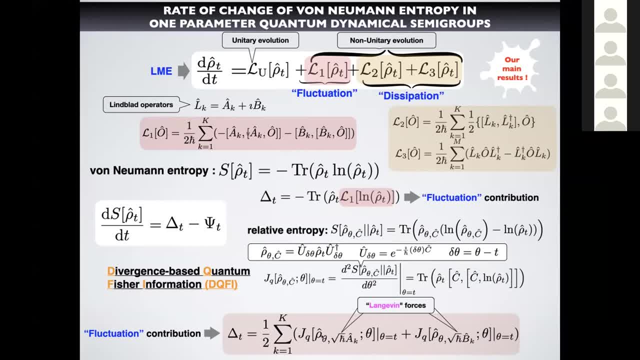 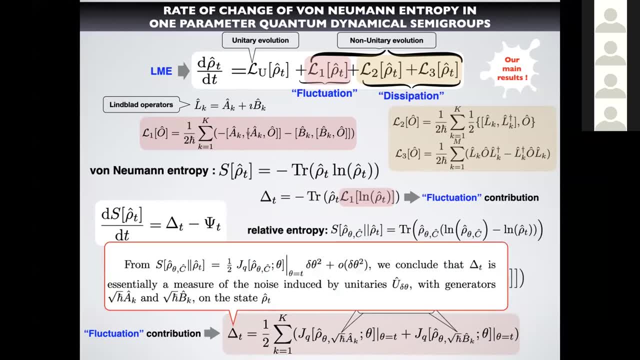 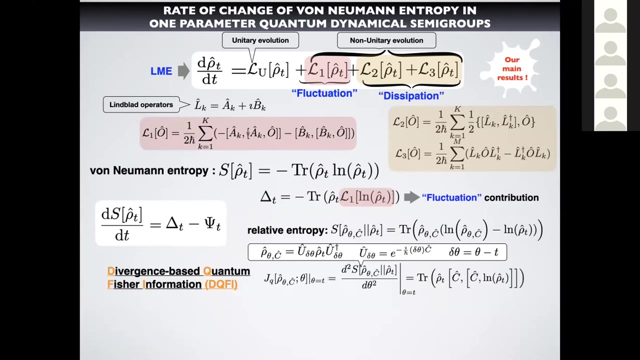 And This Displacement Of The Quantum State Is Can Be Associated With The Quantum Launch Of Forces. This Very Interesting To See That The At 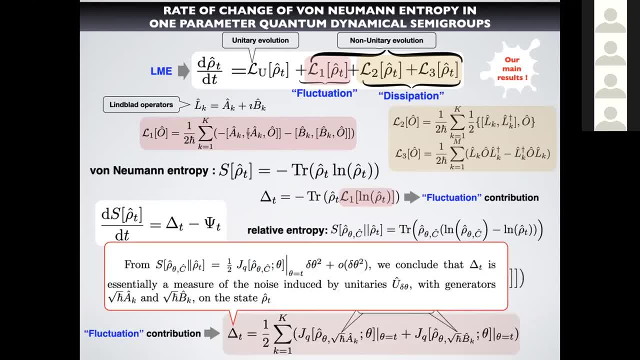 This Diversion, Basic Quantum Can Be Related With The Relative Entropy In This Way. So This Some Of Fish Quantum, Fish Information, Relative, Relative Entropy. 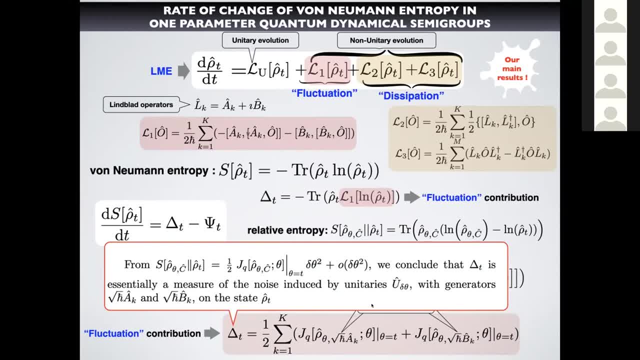 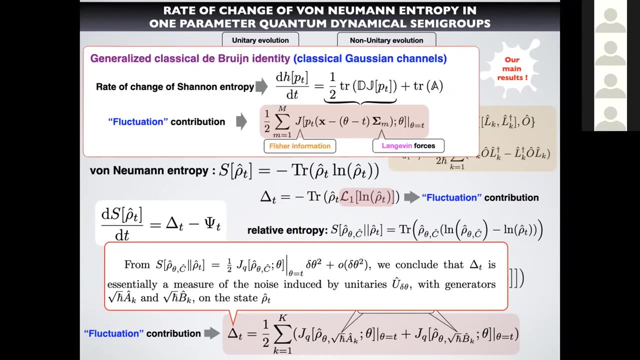 Basis Measures The Noise That This Unit Evolution Is. There Is A Microphone That Is Open. So If We Compare This Expression Here, When The 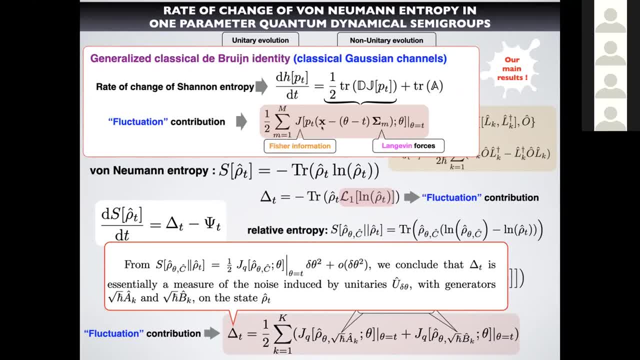 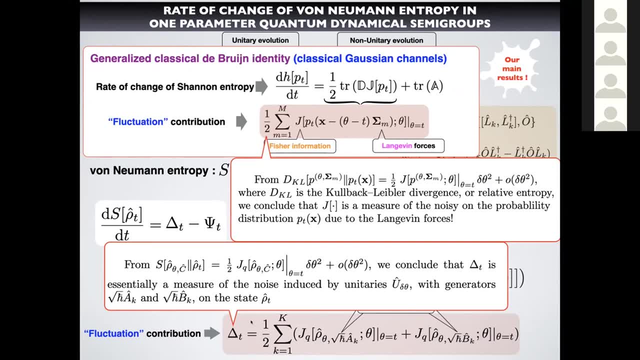 Expression That Appears In The Classical Gaussian Channels, That We Found A One Entropy. Okay, But You Have Also This Part Here. That Is The. 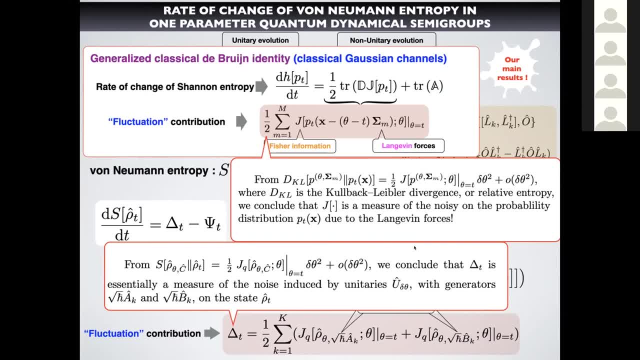 Measure Of The Noise Introduced In The Dynamic By The Launch Of Our Forces Here. Okay, So This Is A Quantum Debris Identity For Any 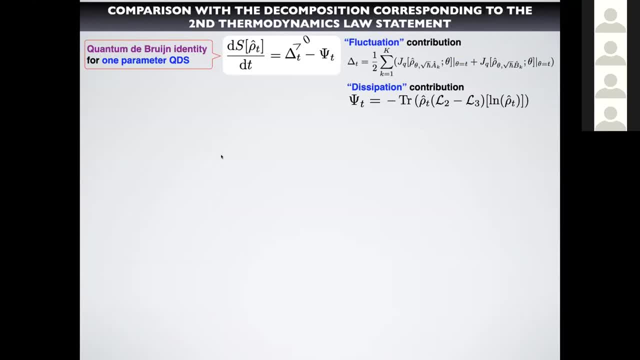 Quantum Dynamical Simulator. Okay, This Is Our Main Result Of Our Work, So Let's Compare How The Equilibrium Appears In A Stationary Situation Arise. 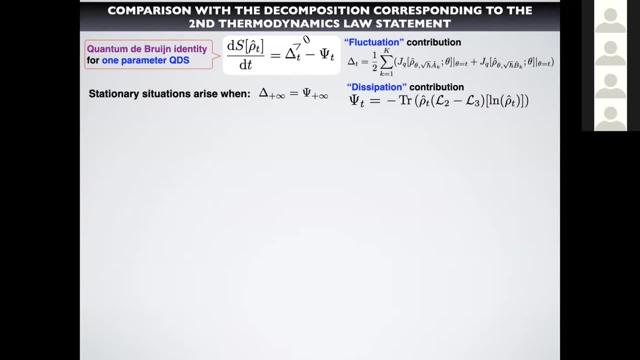 When These Two Times Balance, Because The First Time Is Always Positive, It Can Not Be Zero And In This Situation, In Mass Balance, The Second. 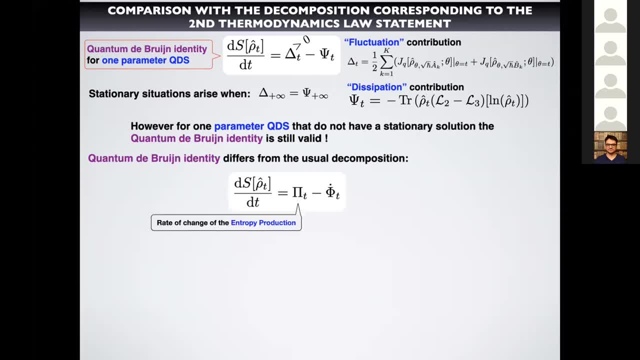 So This Is Not The Same As This And The And The Second Time Is Not This. Okay, And In In The Problem With This Description. 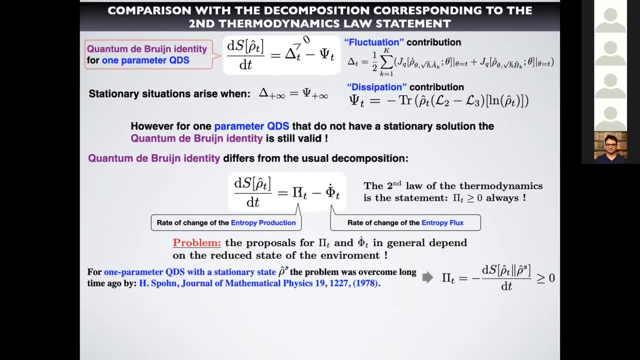 Here Is That For The First Time. For Example, It Depends On Things Of The Environment. Okay, You Can Avoid This Problem And Have An Expression. 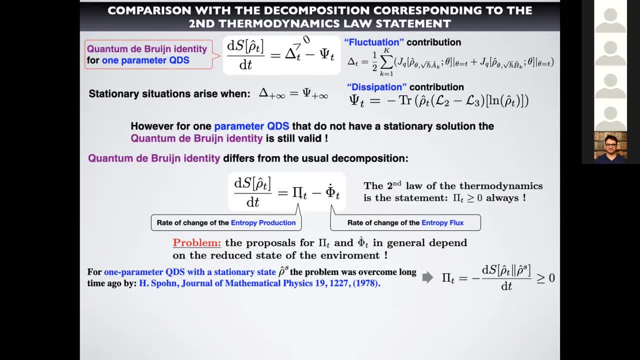 Only With Ingredients From From The System And Performance, But The Spawn And Expression Is This One. Okay, And In This Case, When? But This Only. 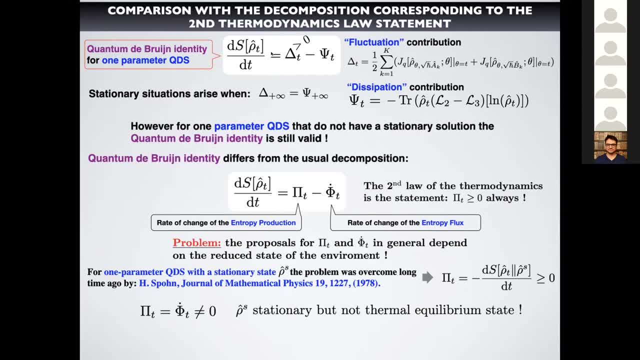 Can Be Done. This Only Can Be Done When The Quantum Dynamical Do Not Have Any Stationary Situation In This Description. As I Said, The 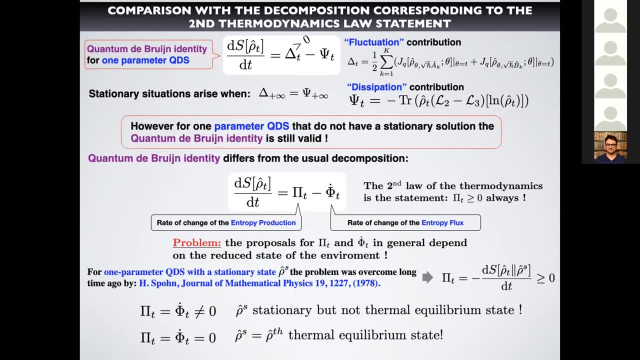 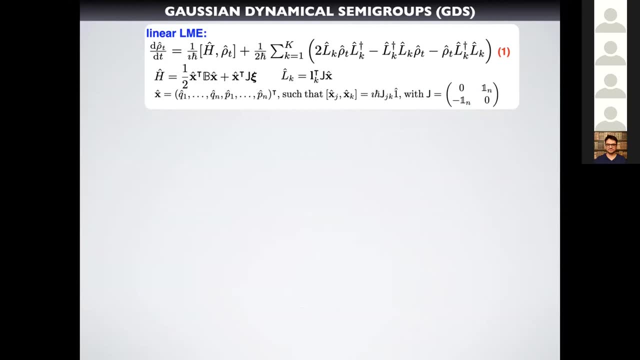 Stationary Situation: Distinguished Between The Stationary Situation And The Equilibrium Terminal Situation. Okay, And We Will See The Routine In This One 呼. 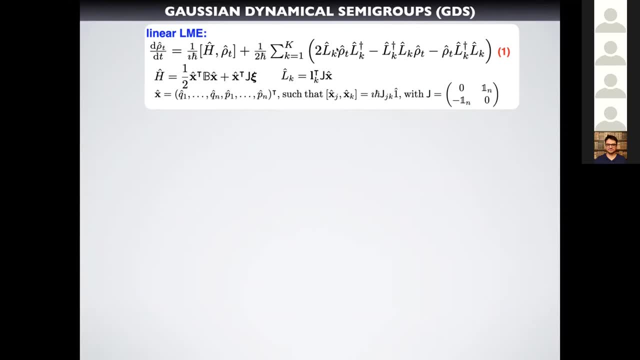 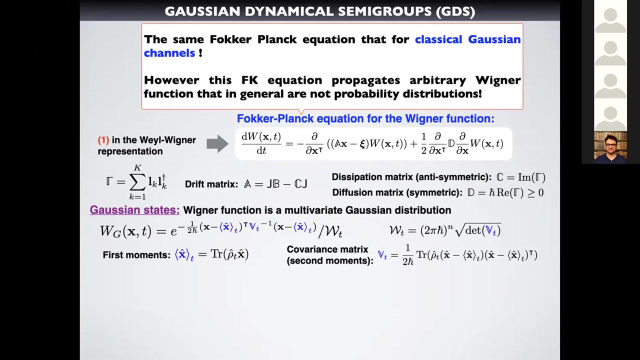 Now En One, As We uh, canonical conjugate operators. okay, these are: yes, you have around five minutes, including the question. the question, okay, so, uh, i will go quickly. so in this case, in for this type of system, the description for the binger function of the system is: verify, the same. 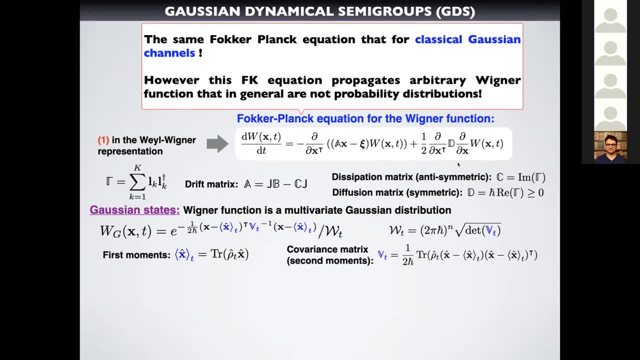 pocket plan equation. that the classical case, but in this case the binger function could be a probability distribution or not, when the this binger function correspond to gaussian states. this is the that are a probability distribution. you have a description, or the same description and the classical case in this case. 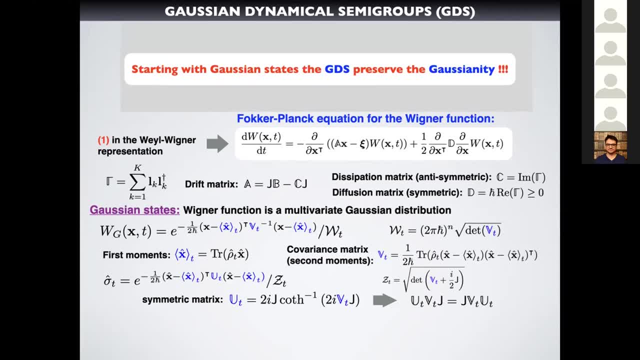 this channel is preserved, the gaussianity. if you start with the gaussian state, then you end up with the gaussian state and in the stationary situation, if you, if the, the system has a stationary situation, the station state is gaussian and all initial states and apps in that. if you start with any state, you end up in this gaussian state. so, uh, let's, uh, i want to. 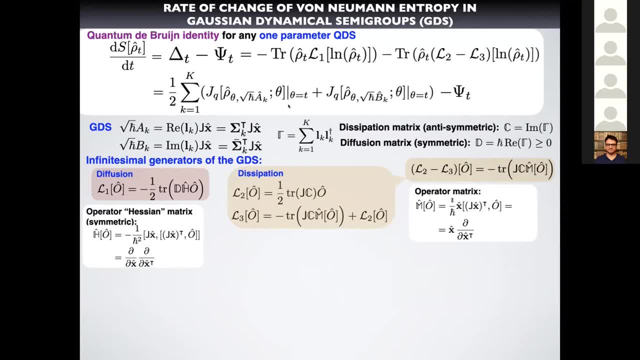 show the quantum diversity identity that we found. in this case, you correspond if you apply this, this is for any quantum dynamical semi-group and to use the quantum, the lindblad equation, uh, you end up with this. uh, quantum degree identity from gaussian dynamical semi-loops. and if you compare, 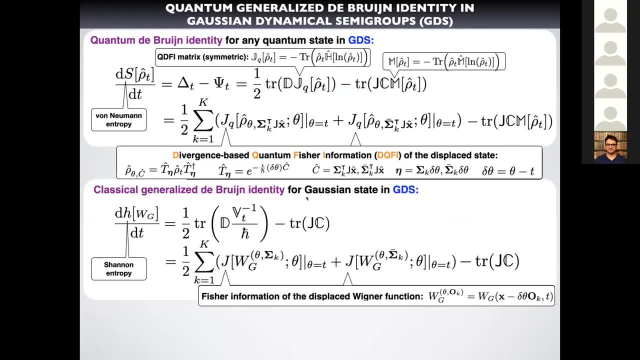 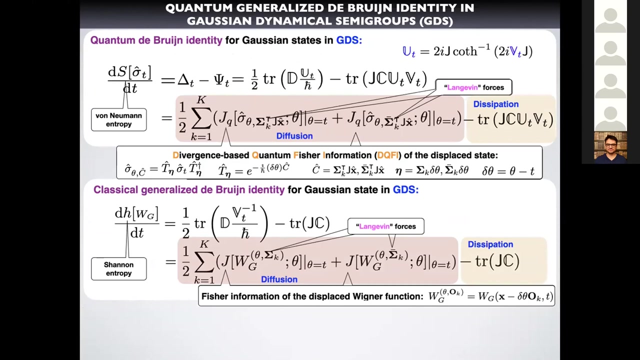 for with the classical case, you see a very similar structure. okay, but uh, here's appear, for example, the, the matrix uh for the quantum uh, division, basis, quantum information. and here appears the classical case. okay, well, let me. but if you, if you apply a, if you start with a gaussian state, that is, 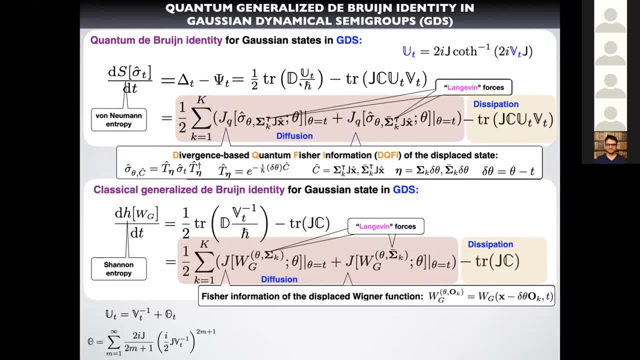 in this quantum division identity. you can calculate the quantum division, basic, efficient information and gives this expression here. and if you compare this with the channel entropy, you see a very similar structure also. but in this case this matrix that appear here and this matrix that appear here are connected and you can. 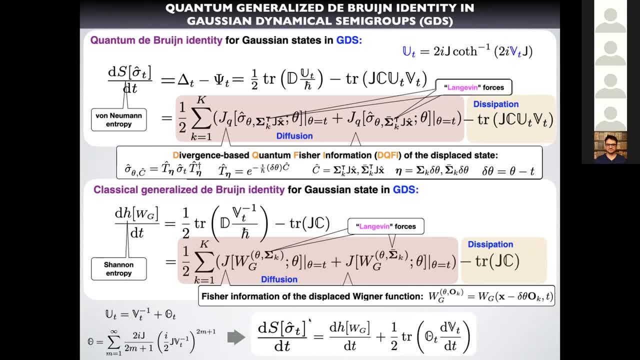 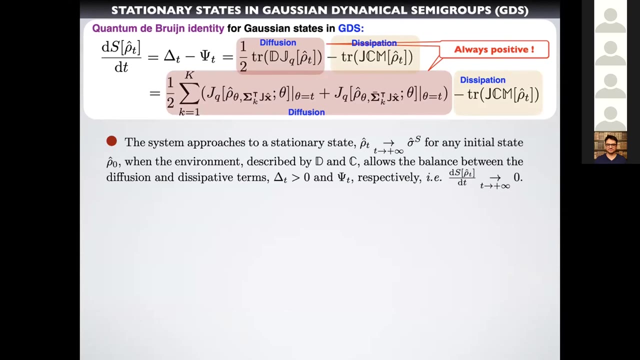 prove this relation. so there is a relation of the quantum division identity and the classical division entity. when you start with gaussian states in quantum dynamic, gaussian dynamical semi-loops. well, in the case, if you analyze the situation, when, when you goes to the equilibrium, the equilibrium 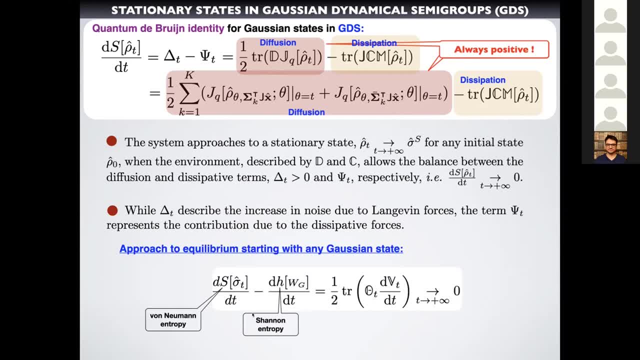 you. you goes to the equilibrium in a way that this difference here goes to zero. okay, so in the equilibrium the monomer entropy, the rate of change of the momentum, goes to the rate of change of the channel entropy and goes both, goes to zero. okay, let me show a. i will. 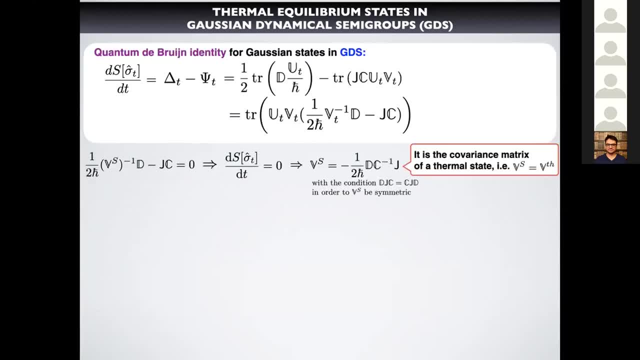 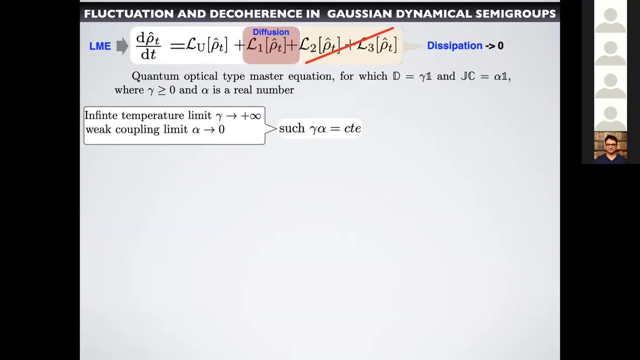 this is a way to to to, to distinguish equilibrium from a stationary situation. i don't enter in this here, i don't have time, but i want to show this last transparency that shows that our the composition of the non-unitary infinite semi-propagator of quantum dynamical semi-loop. 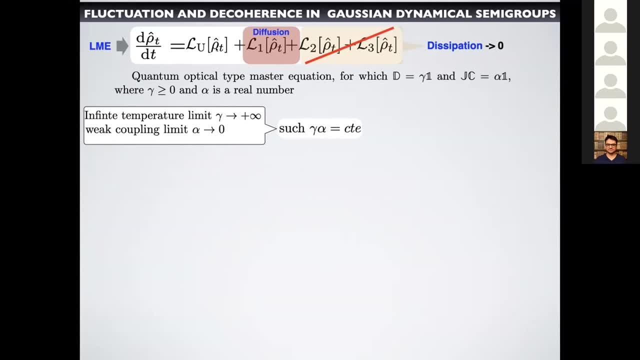 is related with the coherence, and here we have the, the gaussian dynamical semi-group in continuous value system. but and i want to show a, a numerical simulation, but the, the, here the simulation is not associated with a quadratic hamiltonian, because i don't, i, i, you, i use this from an old world and this 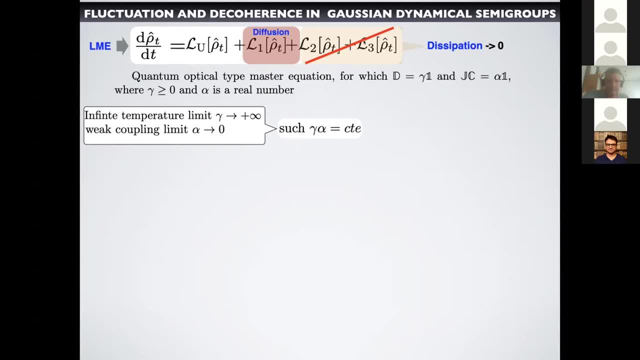 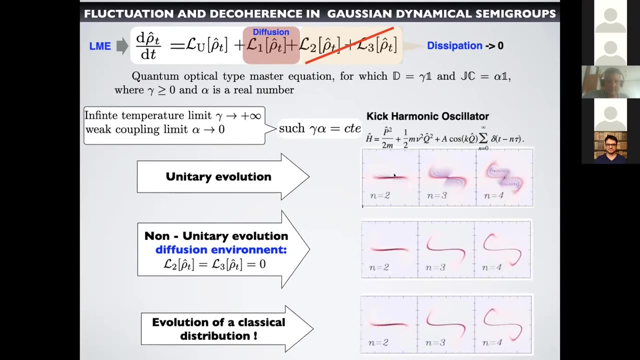 so the, the, the non-unitary part, is the same as the gaussian dynamical semi-loop, but the unitary part is not quadratic, it's a non-linear uh evolution. and here you we see a the following: if you start with, for example, with a gaussian state, 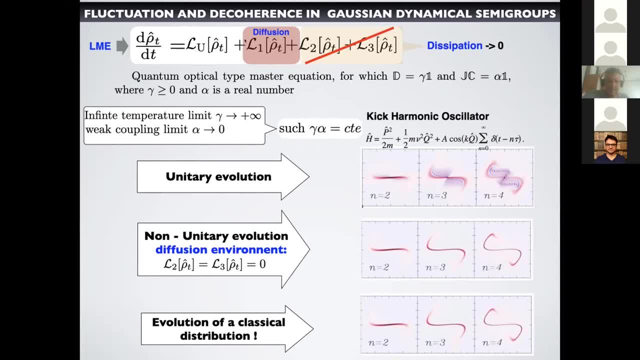 that this is a coherent state without this part. here, this coherent state evolves here with a non-linear key harmonic oscillator, okay, and you see that the binger function starts to show a interference pattern. uh, and here you, we have the, uh, the non-unit of the two, the step of the two: evolution, the unit plus the non-unit. 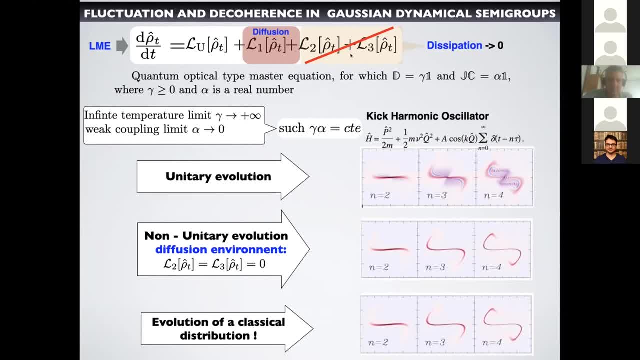 that corresponds to the new university, part of a global dynamical semi-loop. and here in the, at the bottom, you have the classical revolution, uh of uh, not a quantum evolution, and you see that a Crimson, not classes evolution of a quantum evolution, and you see that that are almost identical. 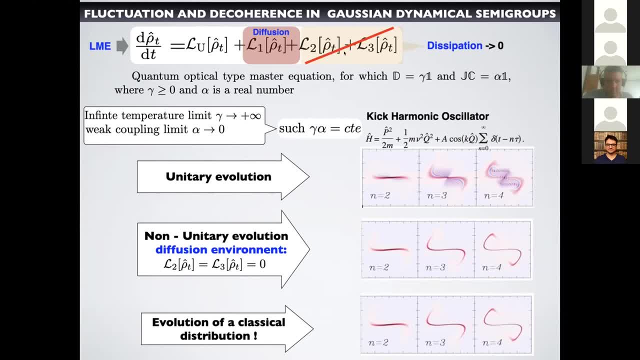 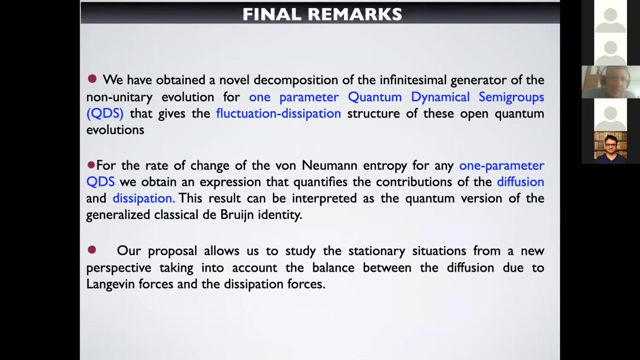 So in this case we used a limit where this dissipative part is zero. So we only have this diffusion part. So this shows that diffusion of this is associated with the gohelins. I'm sorry, Fabrizio, but we are on time. 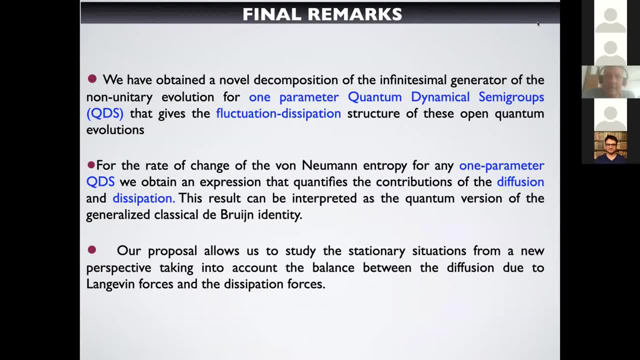 We need to make a break before the session.